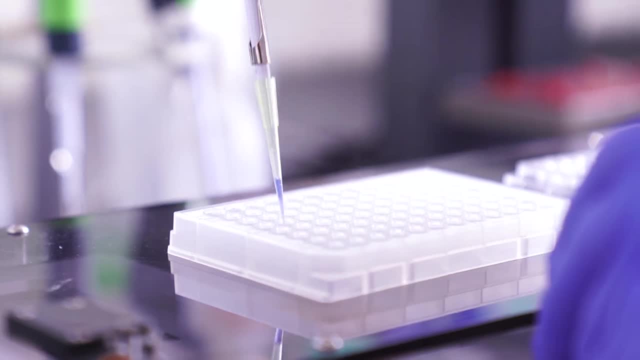 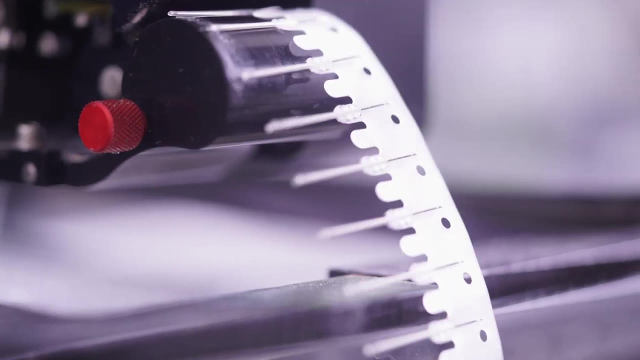 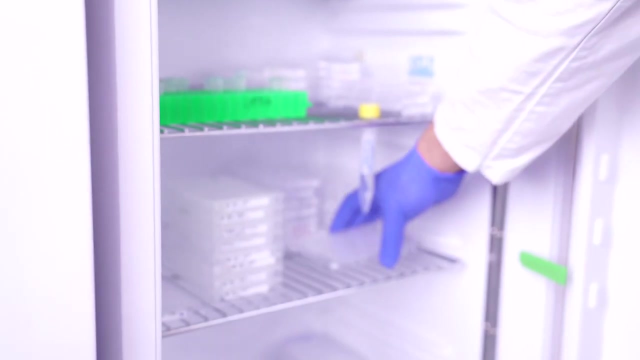 Protein crystals form in saturated solutions that contain many different chemicals. So to increase the chances of obtaining crystals, we set up high-throughput crystallization screens with the help of robots. The mosquito robot pipettes purified protein samples and mixes them with thousands of different saturated solutions at nanoliter volumes. 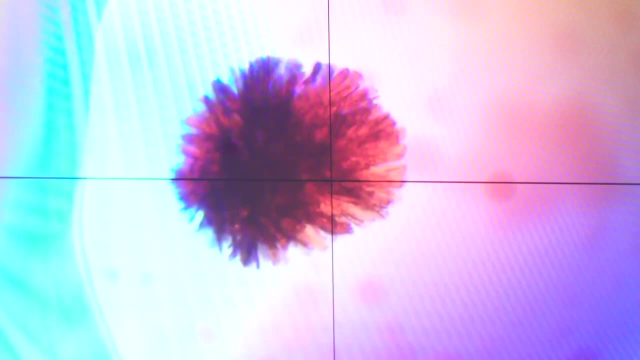 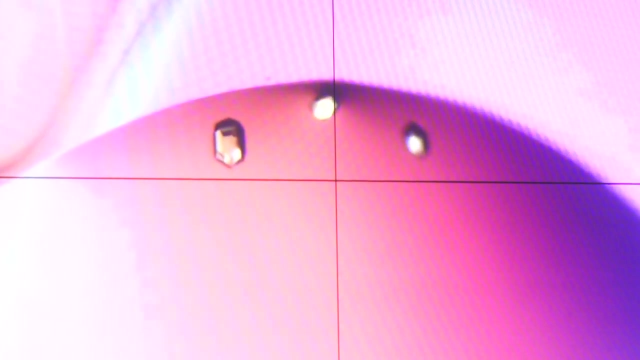 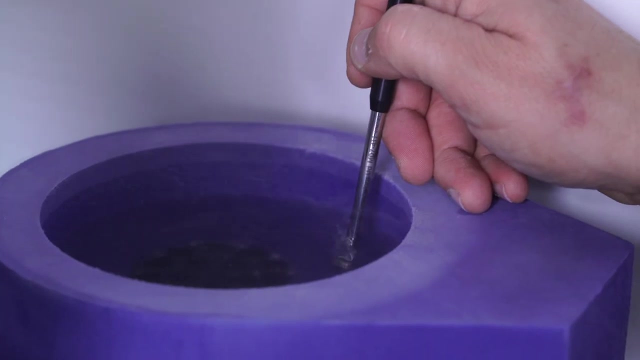 The appearance of crystals can last from several days to months. Protein crystals come in different shapes and sizes. The most promising crystals are cryoprotected, frozen in ultra-cold liquid nitrogen and mounted into tiny loops under the microscope. Then they are shipped for X-ray diffraction analysis to high-end facilities around the world. 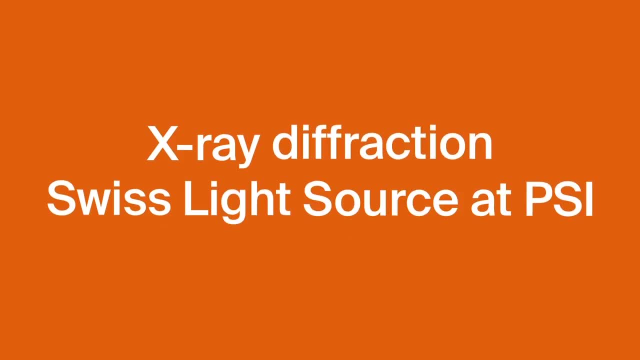 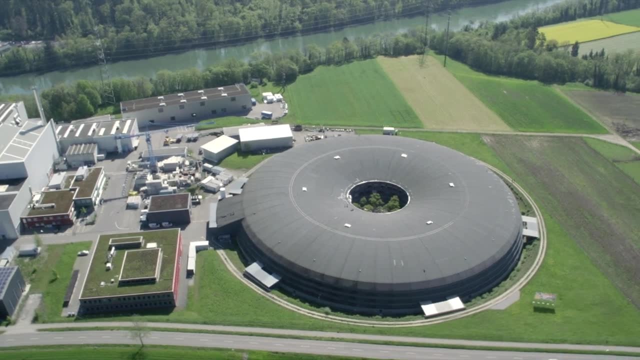 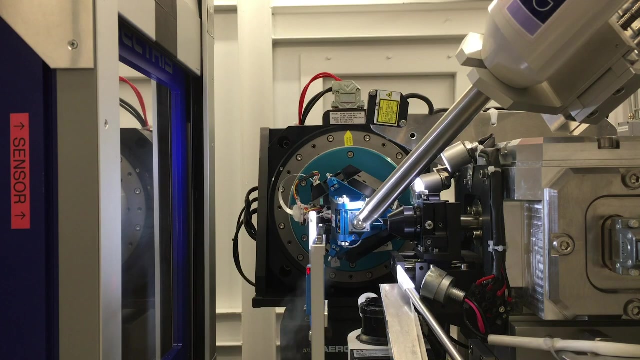 At EPFL, we ship our crystals to the Swiss light source at PSI. This is a very powerful particle accelerator called a synchrotron and is open to scientists for physical experiments. Experts place the crystals in a robot at a specific beamline dedicated to structural biology experiments. 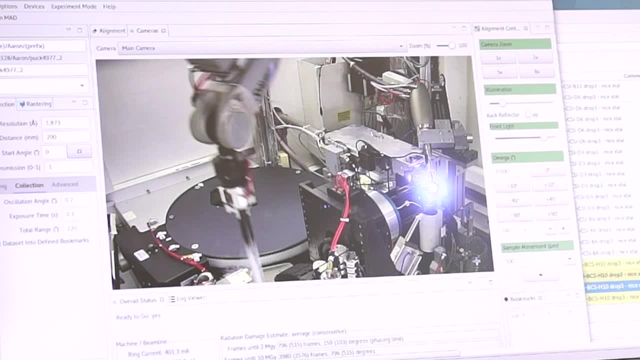 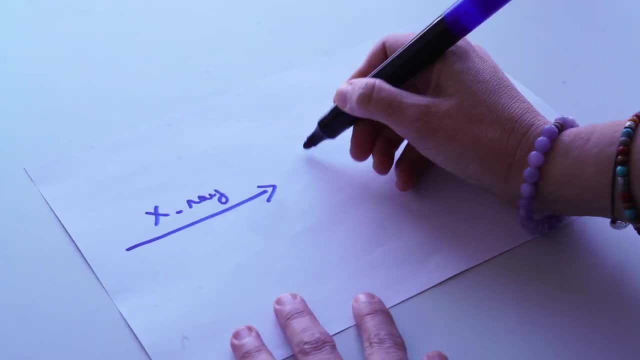 We can actually operate the robot remotely from EPFL. The crystal is placed in a robot at a specific beamline dedicated to structural biology experiments. We can actually operate the robot remotely from EPFL. We shine brilliant X-rays on our tiny crystals and then collect diffracting 2D images for each one. 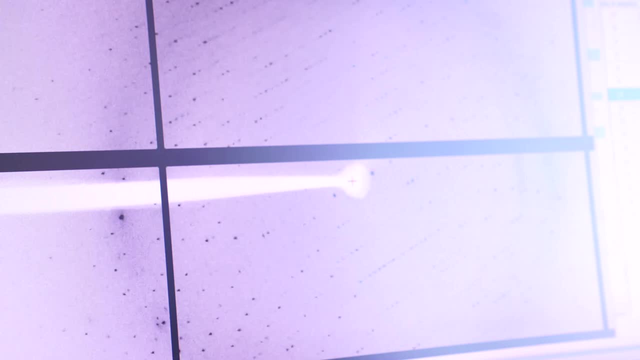 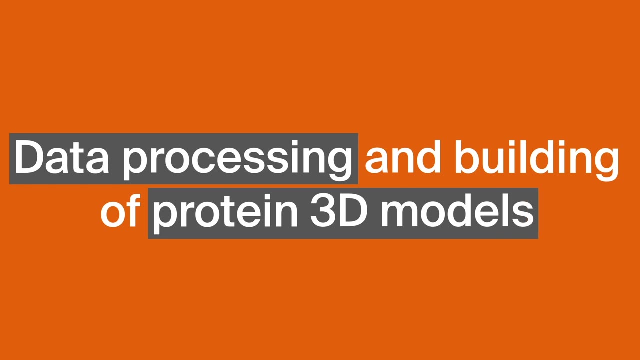 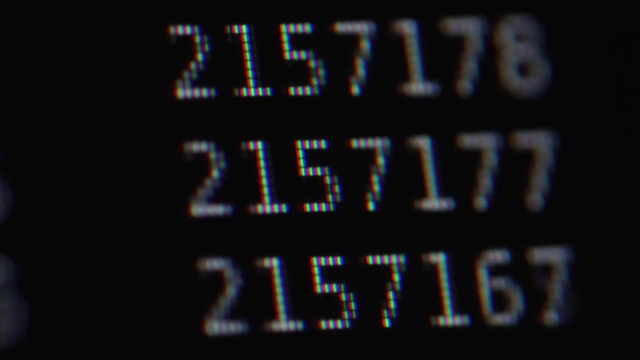 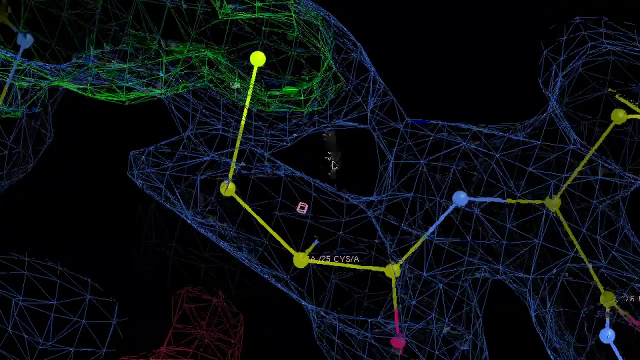 Collecting a complete high-resolution X-ray dataset for each crystal only takes a few minutes. EPFL scientists process and analyze the diffraction pattern of each single crystal to obtain high-resolution density maps, Working with researchers. Working with researchers, we build a final 3D model at atomic resolution. 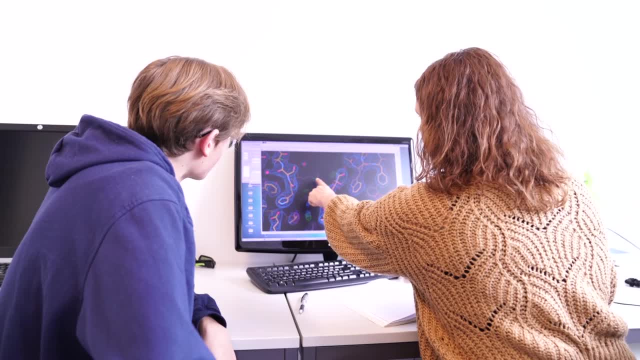 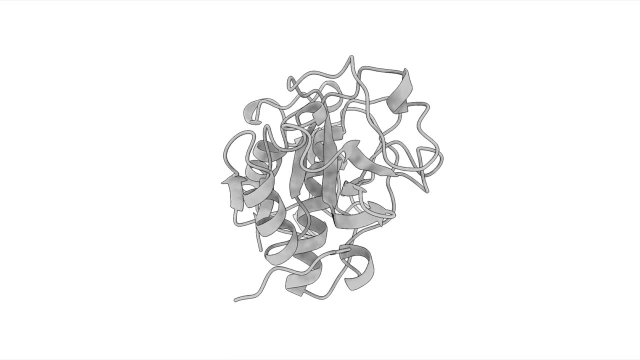 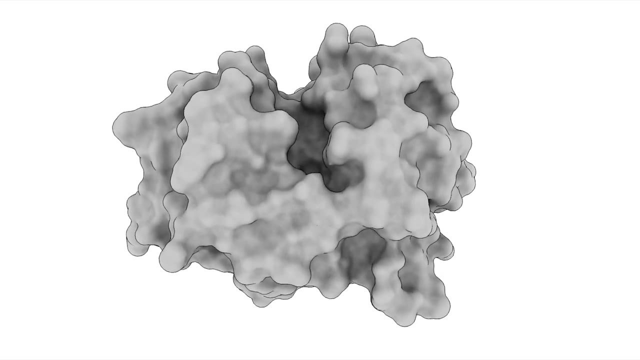 This is then refined, interpreted and deposited in the Protein Data Bank, which contains hundreds of thousands of structures of macromolecules that are freely accessible to the scientific community. At the Protein Production and Structure Core Facility, we support researchers in their structural biology projects. 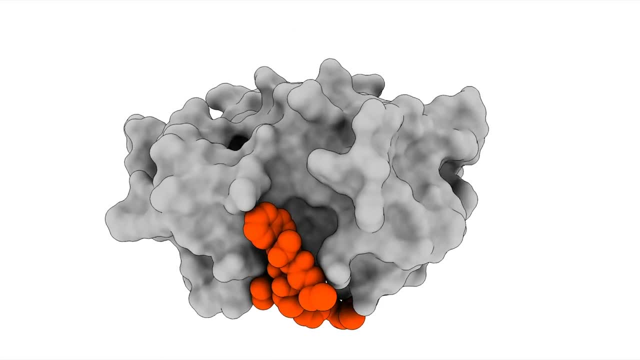 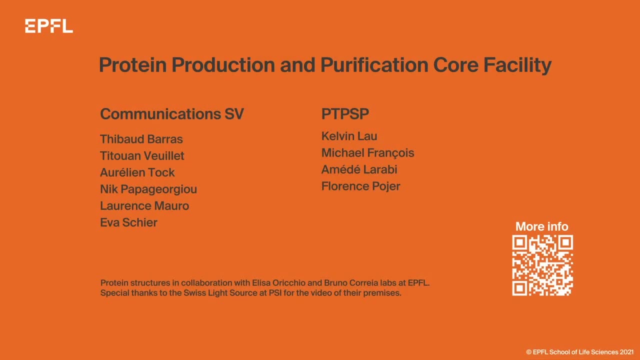 deciphering 3D models of complexes, contributing to a better understanding of biological processes and improving therapeutics. We've built an ecosystem of systems, a network of processes that can be built in a very think-driven way, with ready-made tools and technologies.